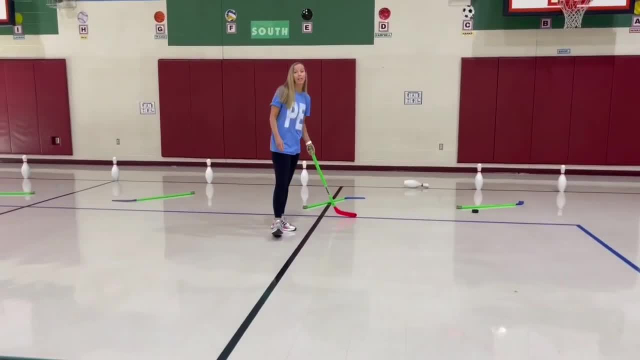 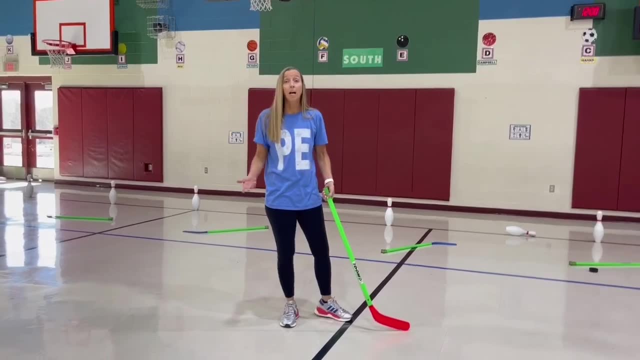 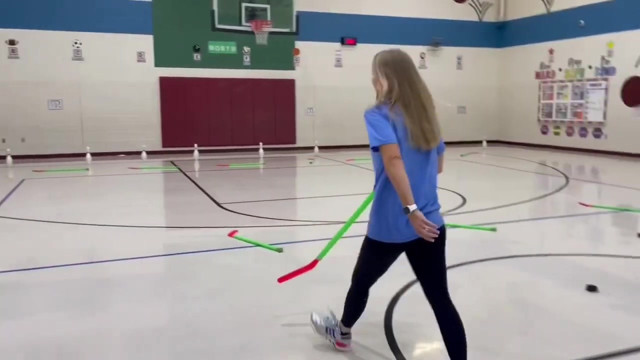 Now they cannot cross over the blue line here, So it's blue line to blue line. They have all that area. When coach blows the whistle and says time, clean up, they're going to take their sticks back where they were, where they started on the blue line here, And they 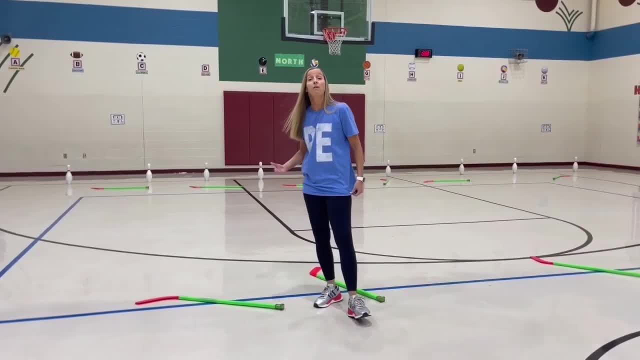 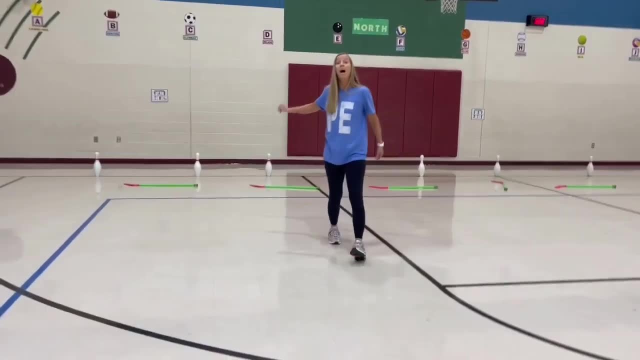 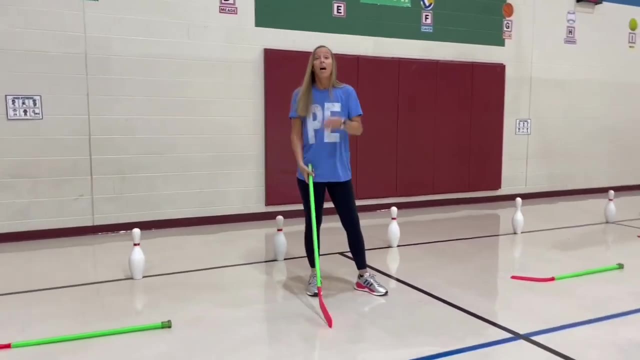 would sit on this line until I rotate. So that is the forward position. Next I have the goalies, And so the goalies position is: they stay behind the blue line And their job is to defend the pins. Now I also. 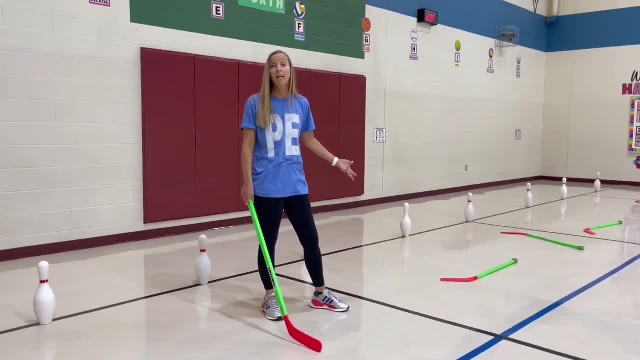 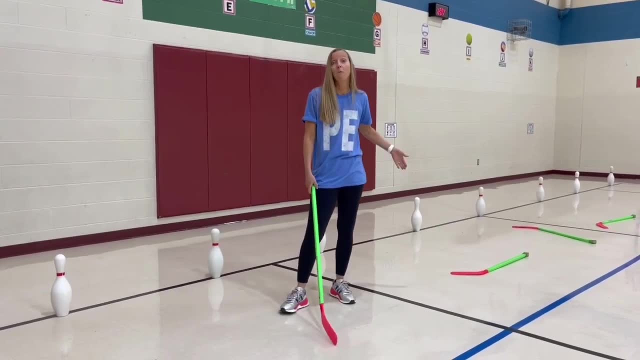 take them, and sometimes I will have six, seven, eight kids back here because again, my class sizes are large But you may not have that number. But so they have to really work hard and work together. So their job is to defend the goals They cannot reach over the blue. 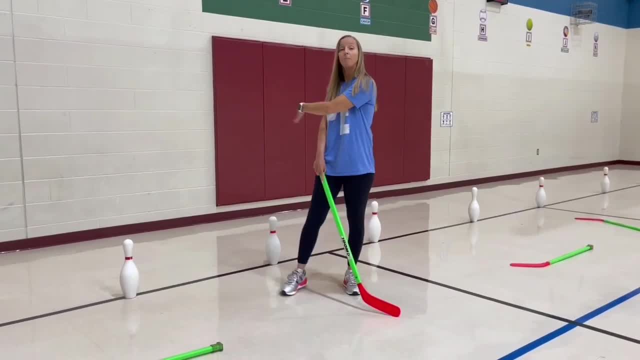 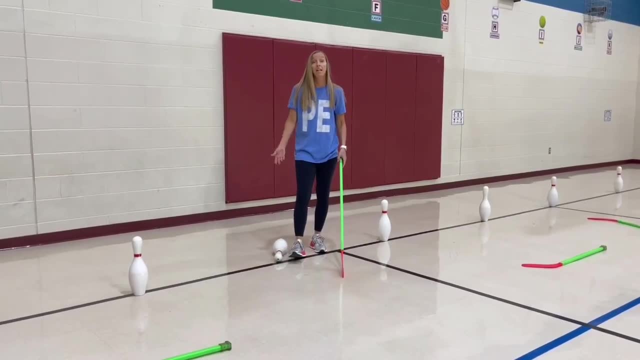 line. They have to stay back here. But any pup that comes back here goes behind the black line all the way to the wall they can get. If they accidentally knock down a pin that counts as a point for the other team Or if 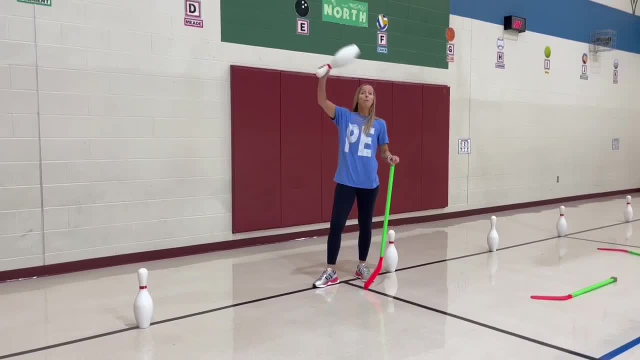 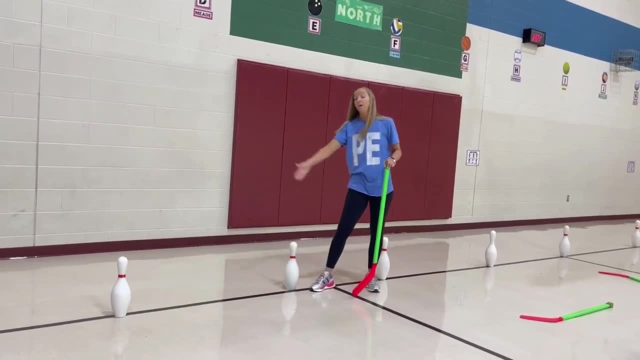 somebody knocks down. what they do is they pick it up, wave it in the air to our scorekeeper. Once they get a thumbs up from them, they set it back up on the black line And I will have little pieces of tape that I put down prior to the lesson to mark. so it's easy. 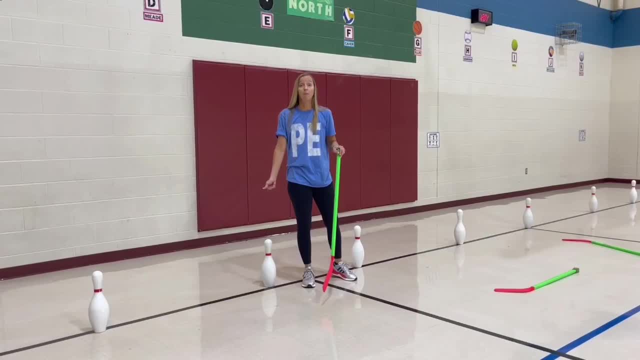 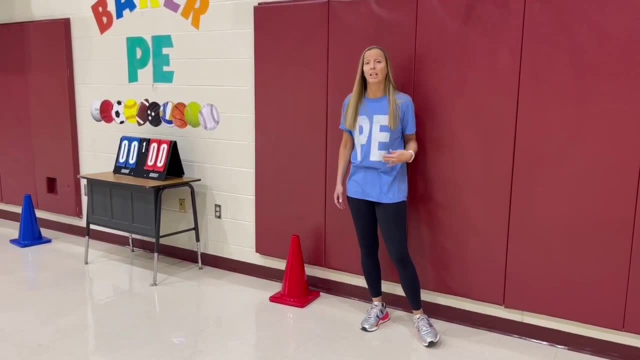 for them to set them back up, So that is the goalie position. The last position is our bench warmers, or our spectators, whatever you want to call it, And they are just sitting against the wall. I only play about two minutes at the most, So that is the goalie position. 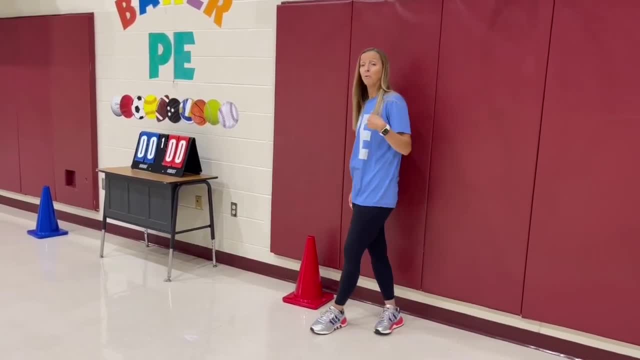 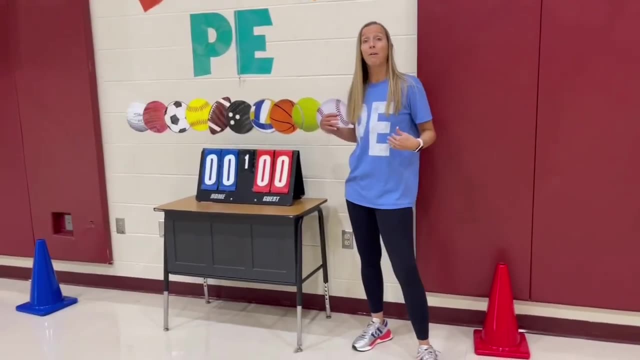 So they are not sitting very long. I also will choose one person that I see doing a good job during clean-up to be the scorekeeper, And I mentioned the scorekeeper earlier. So if I'm on the red team, I'm watching that side down there, because that is our point.